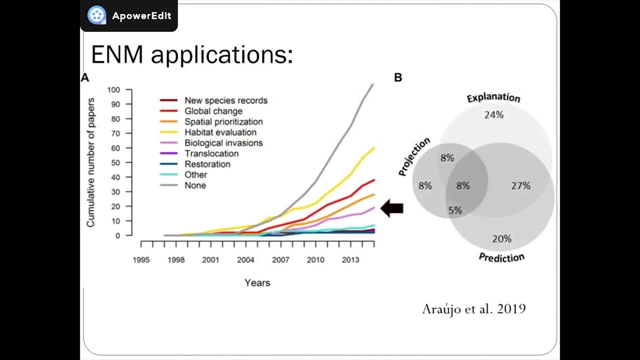 shows the number of publications of knowledge model in different aspects of biodiversity research, including global change, biology, conservation biology- I mean different kinds of conservation biology and biological inference. The number of publications of knowledge model in this field is not so many like global change, biology and conservation. 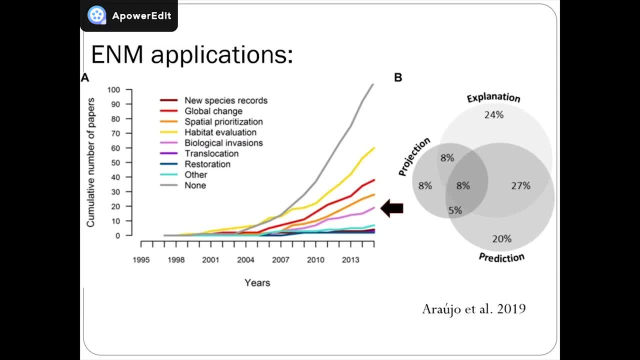 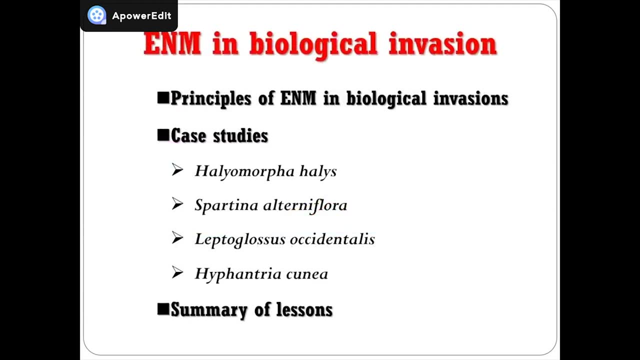 but the number of publications is still rising. I'm going to outline today's presentation. First I will talk about the application of knowledge model in biological envisioning. First I will talk about the application of knowledge model in biological envisioning. Then I will talk about the principle, the theoretical background of knowledge model. 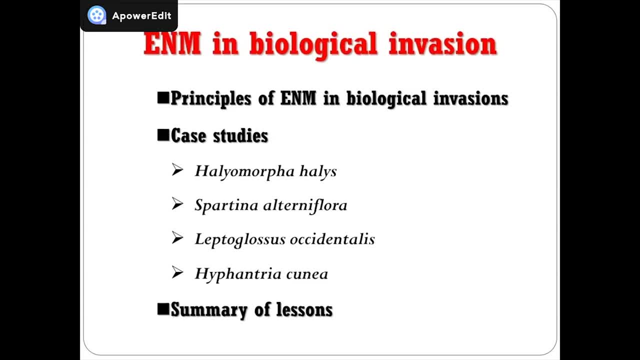 in the universe. Then I will use four species to illustrate knowledge model in the universe. In the end I will summarize the lessons that we can get from the four species, summarize those implications which might be useful for you to develop knowledge model in the. 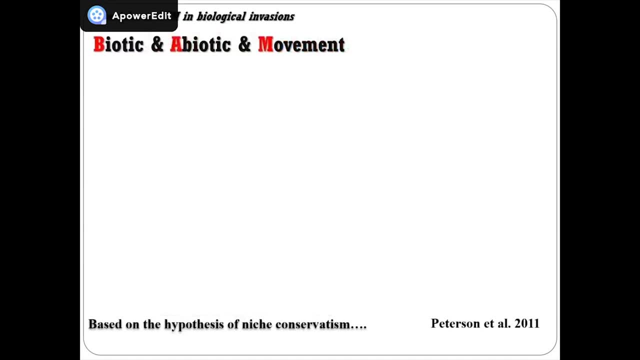 future. Okay, first the principle, the theoretical background. First of all, you need to understand what factors contribute to the distribution, why you can observe the species there but not in another area. Tom Peterson and Hawley proposed the BAM diagram. They used three circles to describe the 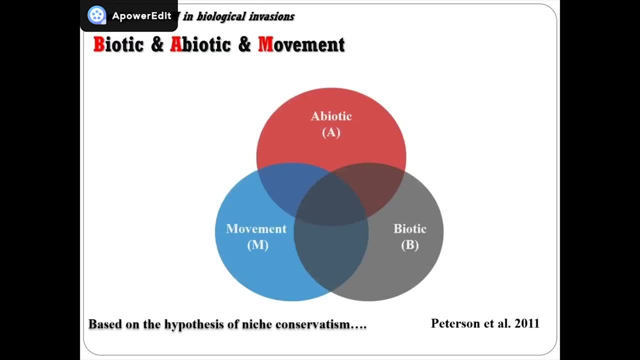 distribution which is including apoptic, biotic and movement. Imagine when you observe the species in a field. when you detect the species there, it must fall into the overlap of the three circles. First, this area must fall into the apoptic requirement of the species. 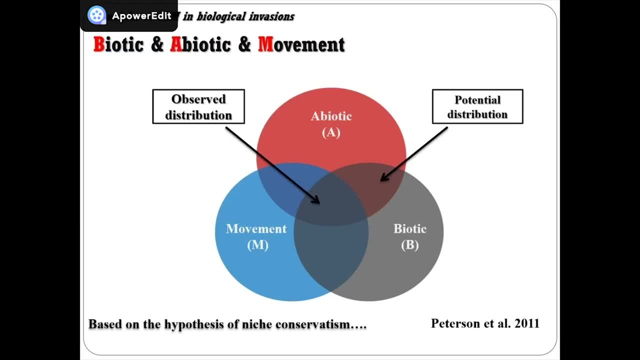 Also in the community. the species can survive, can develop. can develop means that the biotic interaction is good. it's okay for the species to survive. So this area also falls into the movement area. it's accessible. this area is accessible to. 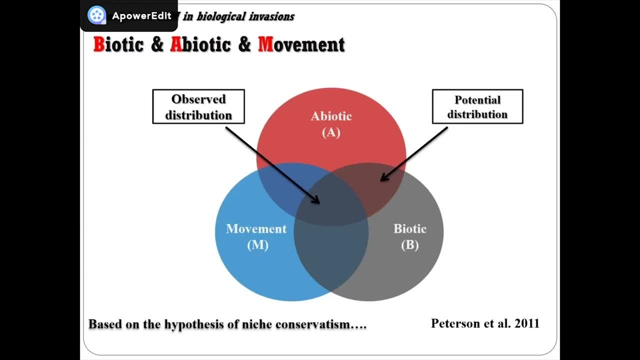 a species. that's why you can detect them there. The overlap of the three circles represents the real-life distribution or observed distribution. There are overlaps between A and B but not M, which means that these areas are suitable for the species, that the species can survive there. 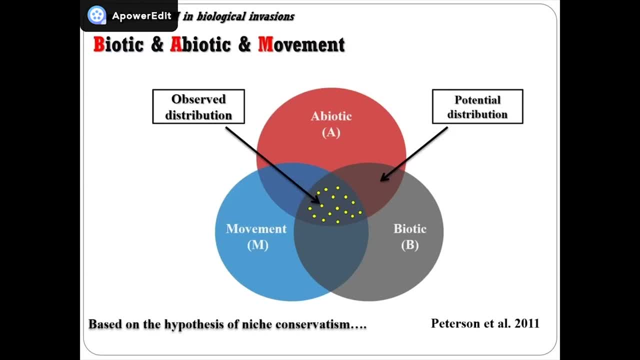 but the species haven't- i mean moved there. All those areas are not accessible to a species. We call this area as partition distribution. Keep in mind this hypothesis based on the niche conservatism I'm going to. I'm not going to talk this topic here, but I will mention it in later. 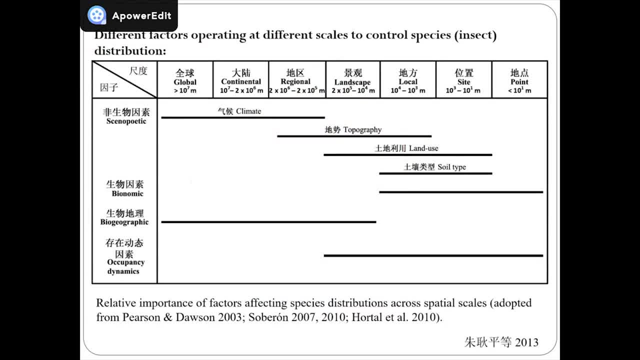 In microecology there is a classical conclusion that different factors function at different scales to control species distribution. Usually climate factors. they are function at broader scale, like global, continental, where those biotic interactions that they function at a relatively small scale, including local site. there are also other factors. 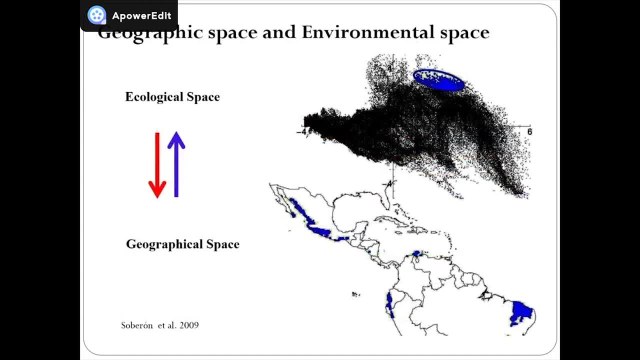 So in this slide you need to understand the relationship between geographic space and environmental space. So in the up figure that is the environmental space, x-axis can be treated as the temperature, y-axis can be treated as the precipitation though the blue point. I mean the classes of blue point. 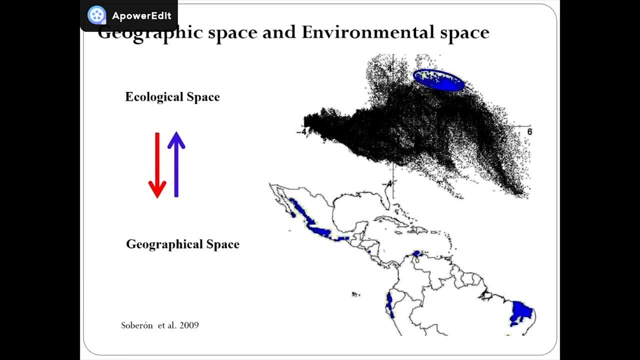 in the environmental space, their projection into the geographic space can be separate. I mean so, which means that the cluster in the environmental space, their projection in, I mean back to the geographic space, those points can not, might not, be clustered. They can be disjunct. 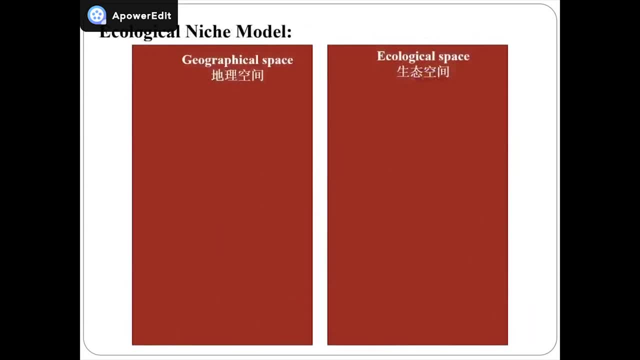 or separately distributed. So niche model fits the model in the geographic space. They use the environmental variables that are associated with the point, which I mean manifest as latitude and longitude. They use those variables to calculate the requirement of species or to calculate the niche. 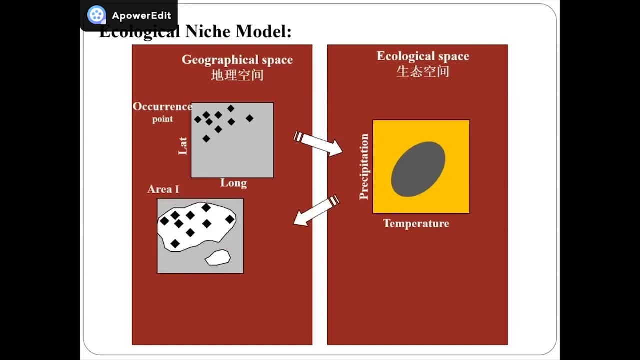 These calculates the niche can be. I mean project back again to the geographic space. They can project it to an area where you have fixed your model or you can project the established niche to another space. Here are the issues of transferability I will talk about. 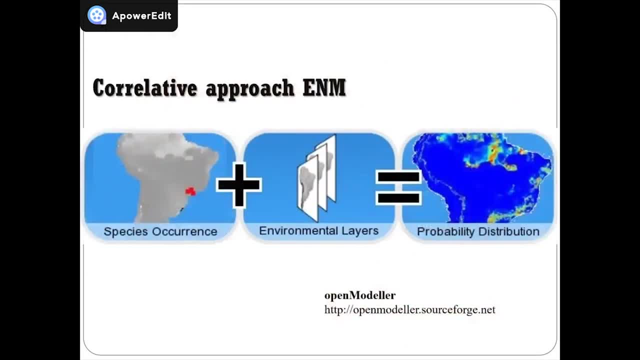 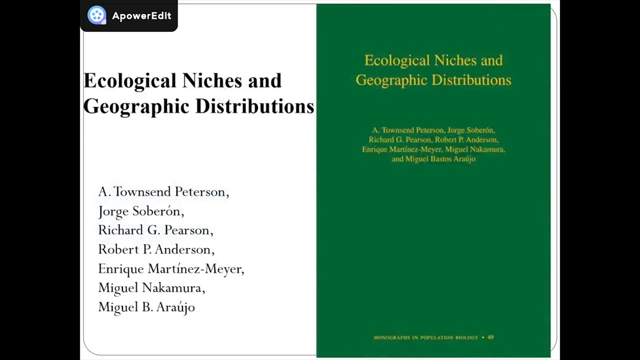 this issue later. So this correlative approach of each model is very simple. They use occurrence and environmental layers to estimate the partition distribution. If you want to learn much background of each model application, take a look at this book Ecological Nature and Geographic Distribution, which is simple and easy to follow. 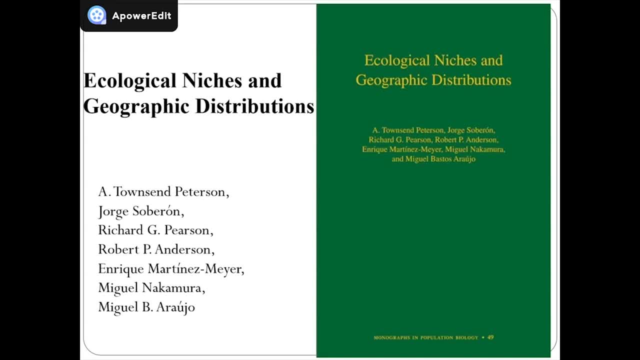 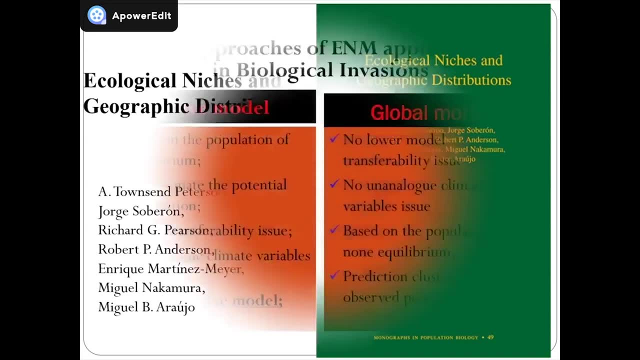 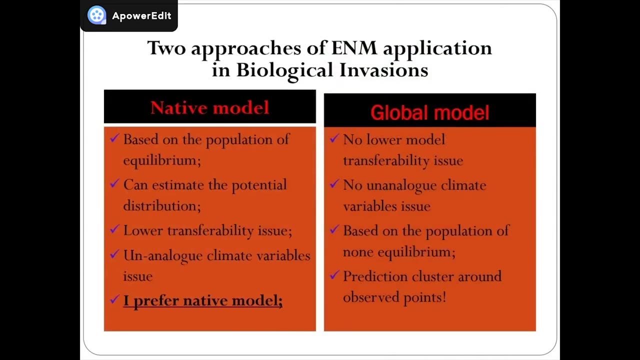 Even you have no idea of biology, no idea of geography, you still can understand the theoretical background, the principle of each model. There are two approaches of niche model application in biological invariants. One is the classical native model approach, which uses occurrence in the native area. 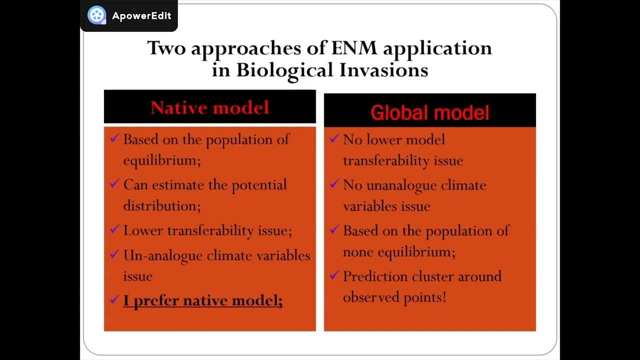 and the other approach is the global model approach, which uses both native and introduced points, I mean uses the pulled points, to collaborate the model, So they have an advantage and disadvantage. For example, the native model is based on the population of the equilibrium. 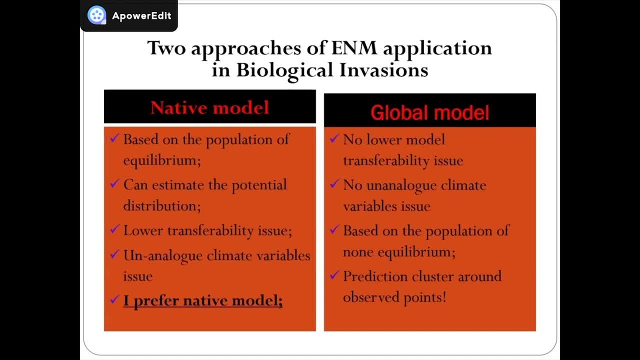 Which is the conception of the niche model application. It estimates the position distribution. But native model have two disadvantages, which is very important, Like low niche model transferability. I mean the native model prediction, you know- introduced error, Their prediction rate is very bad. So they have also analytic climate variable. 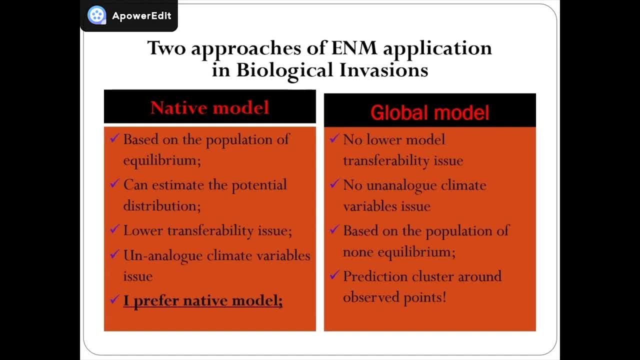 issue, which means the variables are beyond the model fitting errors. The variables are novel to the model projection in the introduced errors. So global model, they didn't have those kind of two disadvantages. but it's based on population of net equilibrium. 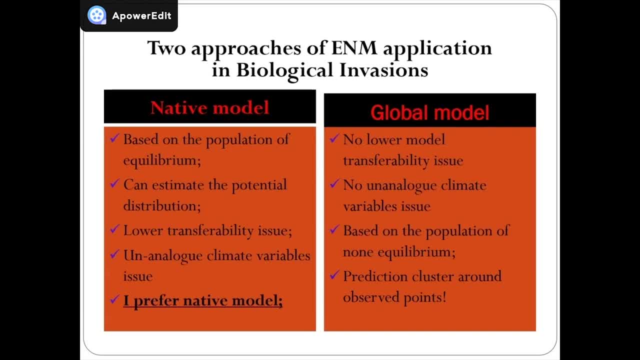 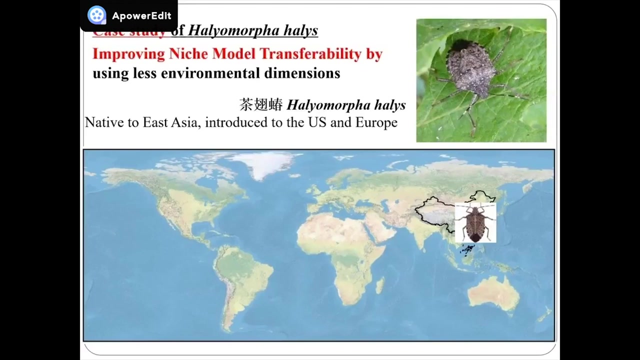 Also the predictions of global model. they have a problem that is usually the prediction is clustered around your observed point, which is very useless in your vision biology. So I prefer the native model approach. I think about Halema Palace. This stink bug is native to East Asia but has been 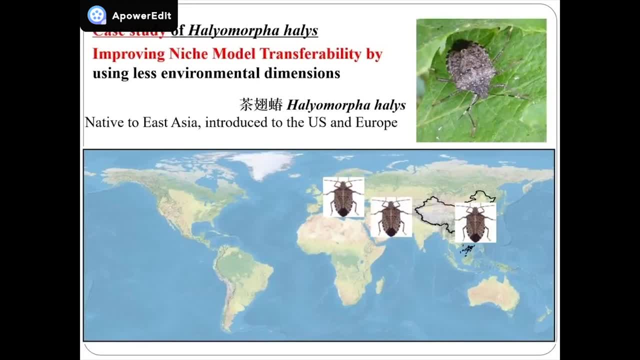 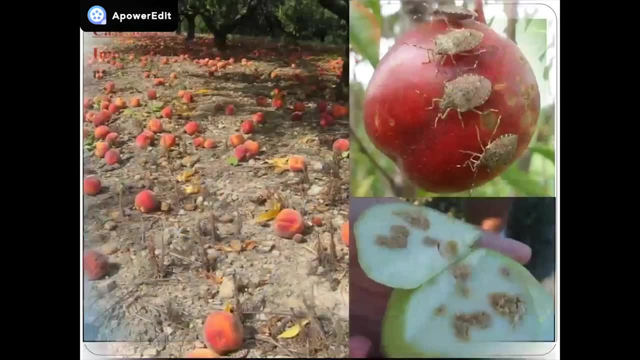 introduced in Europe and North America. In East Asia it is not a serious- I mean pet, it's not a serious problem. But in the West, especially in the Middle Atlantic area, it is a serious problem, especially for the first trees. 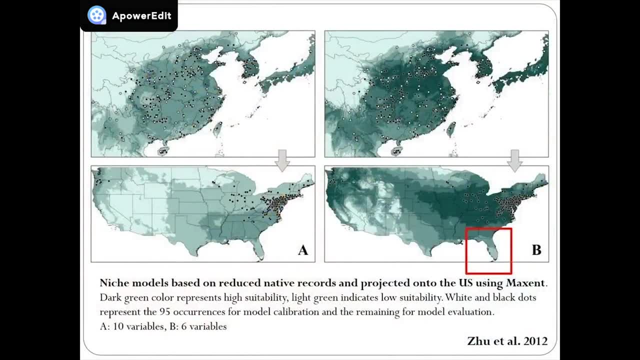 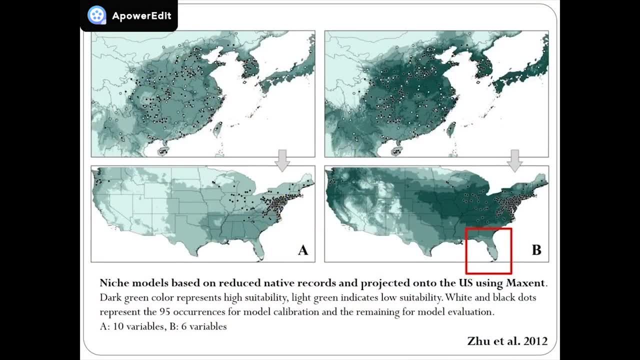 East Asia and transferred it to mainland US. I use two environment dataset. one is using 10 variables, the other is using six variables. left side- A indicating mode will collaborate in East Asia using 10 variables, while the right side, the B indicating model, will. 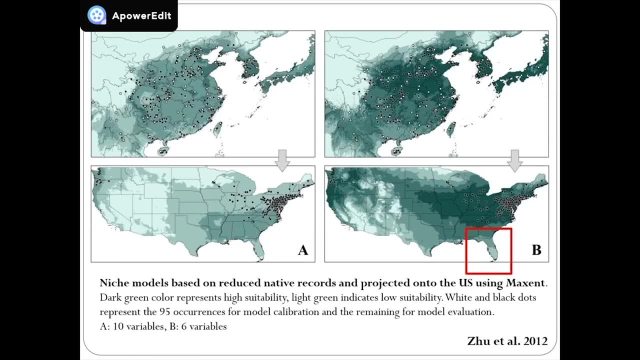 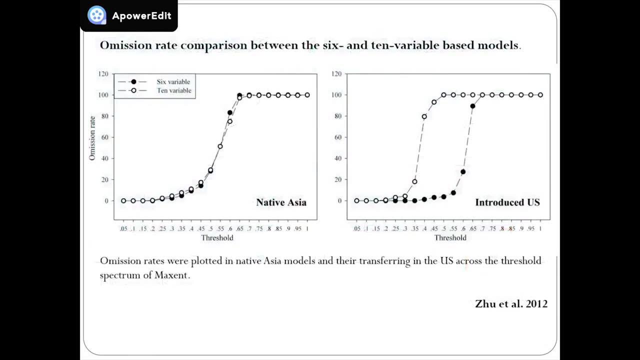 collaborate in East Asia using six variables and transferred to mainland US. from this figure we can see that the model based on six variables shows much. i mean get much better performance. take a look at the omission error. we cannot see any difference of the omission error in the native 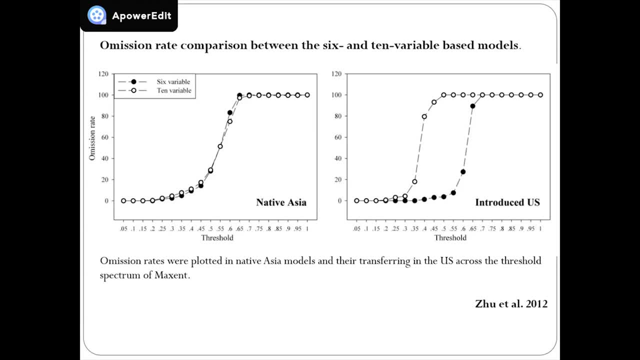 error. but when the model was transferred onto the mainland us, we can see that the model based on six variables showed much lower omission error- those black circles- and compared to the model based on the 10 variables. so this, this result, showed us that it's especially important to think about 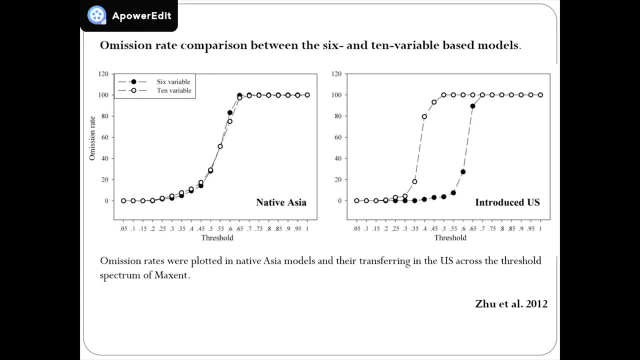 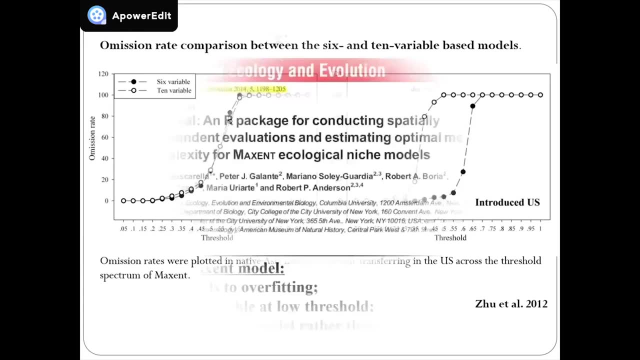 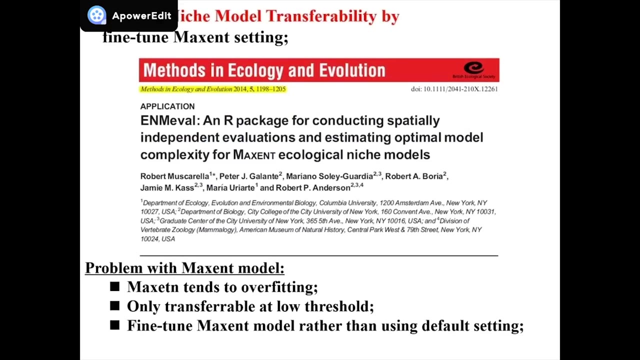 dimensionality, which means how many variables you should consider and what kind of variable you are going to select. it's very important. on model transferability issue is my mixing complexity. maximum is so popular but we find that the company it will recognize that maximum has some problem. 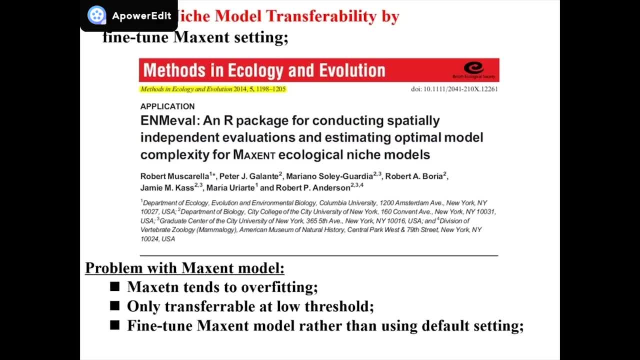 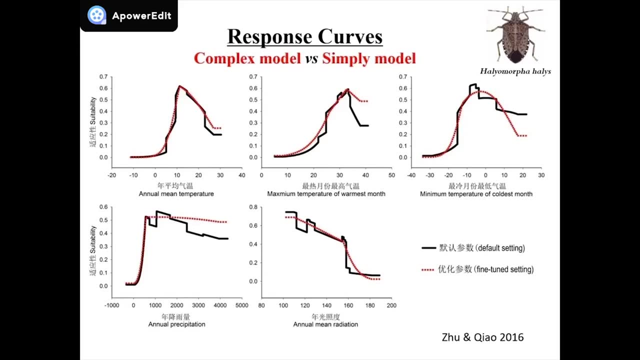 like in the 10 to over 15, they are only transferable at the low threshold and the fine-tuned maximum model setting is much better than the default setting. i use this think bug i. i use the arc to refine the model setting and compare the response curve with those default settings. 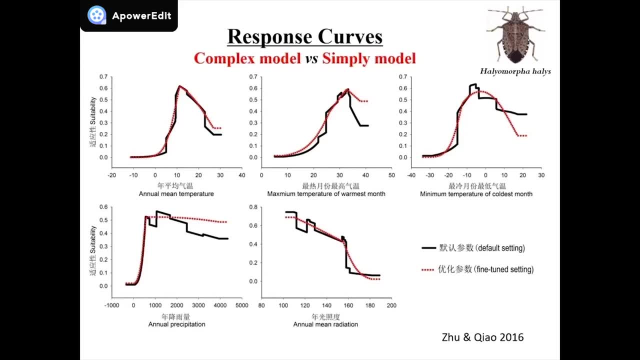 so from this figure we can see that the fine-tuned setting- i mean the model predictions, their, their response curve is much smoother. those dotted red lines is much smoother than than than a response curve based on the default setting. so model based on this, i mean based on the front tunnel settings. 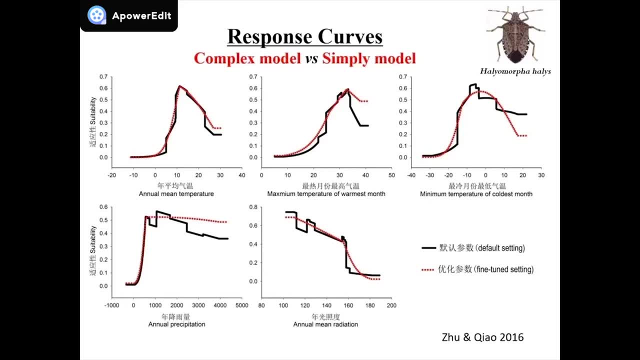 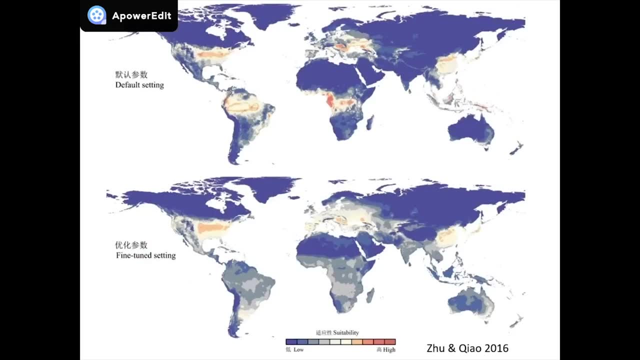 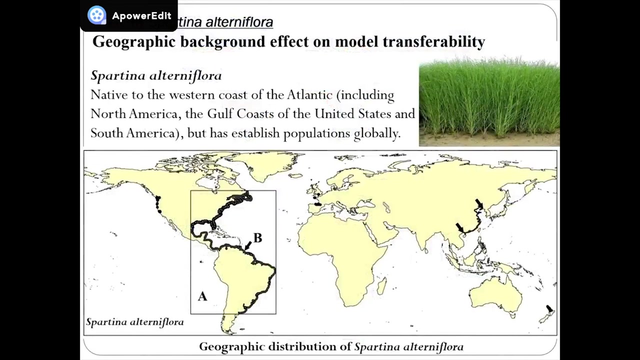 suggests that we are approaching, i mean, the fundamental niche, which is much transferable, so their special predictions is also different. so especially i mean based on default setting and the fine-tuned setting, especially in the silent hemisphere. the second case study: i use: uh assaulted, uh assaulted, a cold grass, which this cold grass. 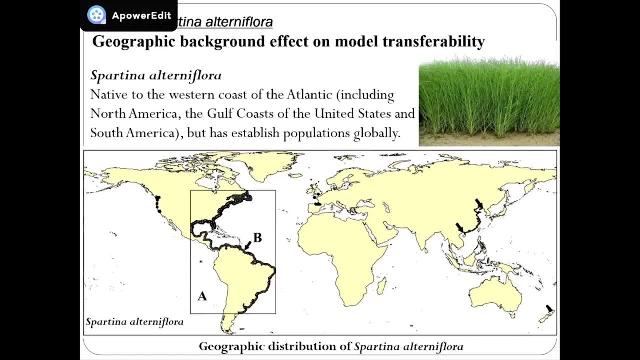 it's uh, they have very special, very featured distribution because they are only distributed along the coast, they cannot display into the inland. so here i collaborate the model based on the coastal area and based on the squared area. so from this example i show the importance of the 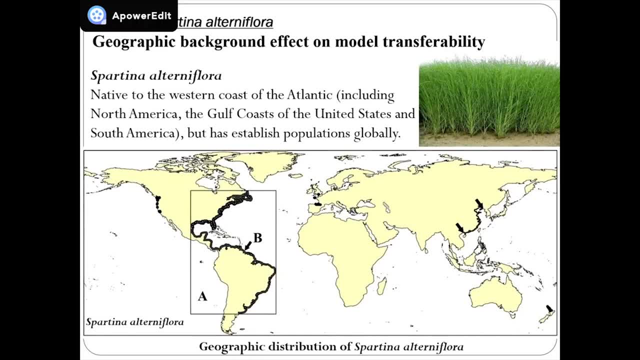 geographic background in each model predictions. i collaborate the model in a native area in- i mean across north and south america, and transfer model onto the eastern area to show the model. to compare the model performance. it's similar to the former stink bug, so based on the squared 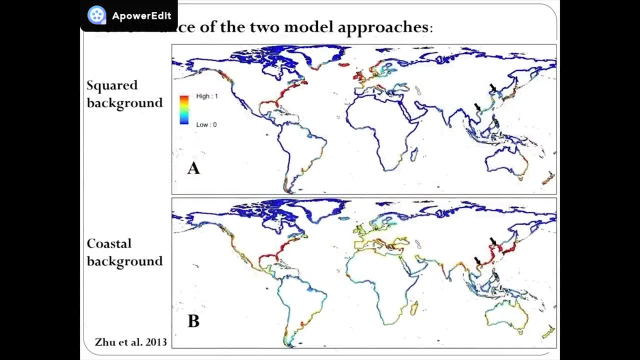 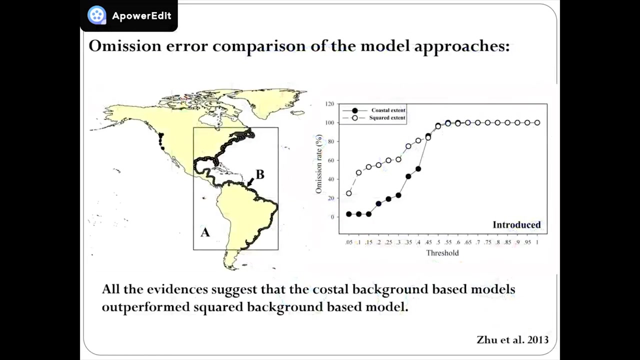 field to capture, introduce the- i mean distribution of this called grass in east area. but model based on the coast ground showed much better performance. take a look at those two- two blacks, black arrows that show the current distribution of this called grass in israel. the importance of model of accessible area in model predictions. 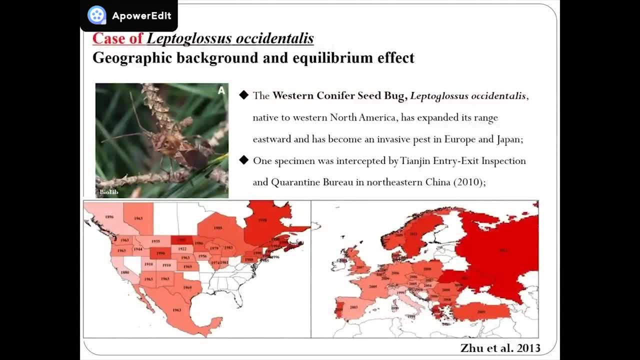 in the. in the third example i'm going to use the western content for city bugger to show the importance of geography, geography background and the equilibrium states. so this species is native to western north america but has uh. it starts to expand its population in early 19. 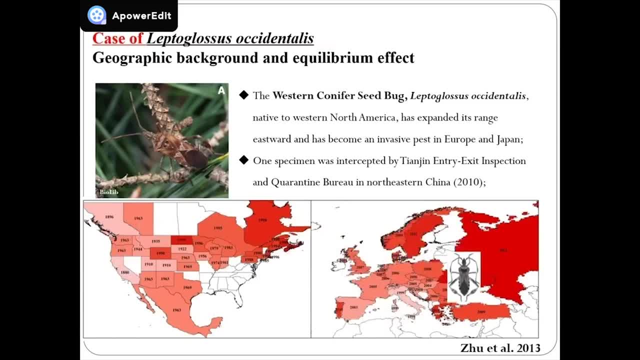 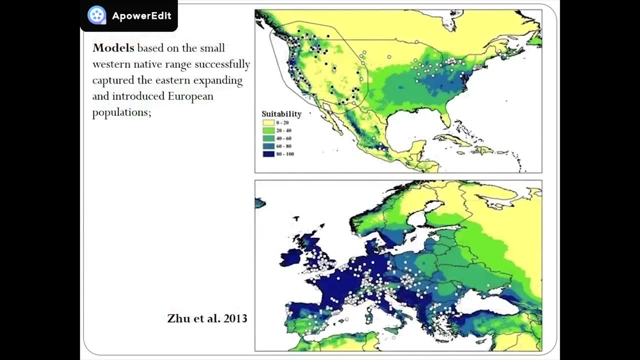 and become an introduced species in europe and japan. it was also intercepted by in china. so model based on the classic native approach, based on a small native western range, successfully captured the eastern expansion population and also introduced the population in rio. that's amazing of the native model approach. 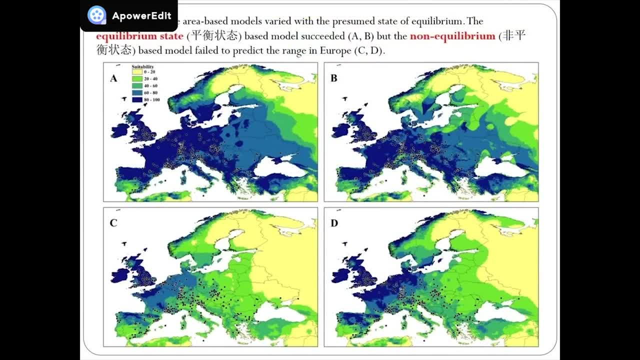 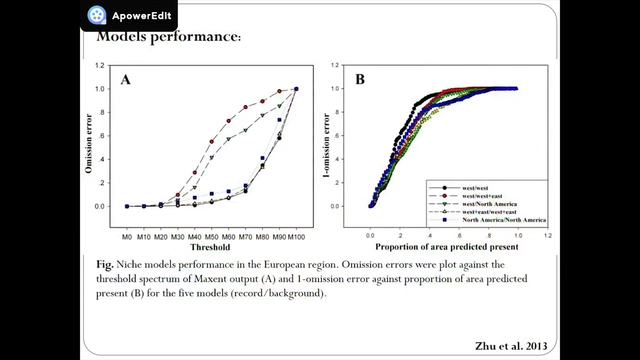 based on large era, based on the whole node and now based on whole american, north american, i mean- area. it's varied, based on its varied, with the presumed states of equilibrium. So based on the equilibrium states that the model successfully captured the population in Europe, Where the model based on non-equilibrium states, they are fueled to capture the predictions, to capture the range in Europe. 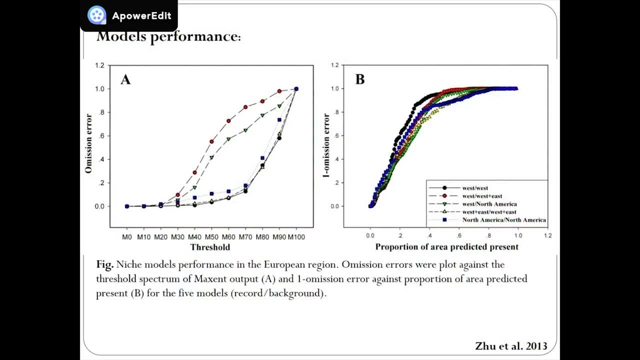 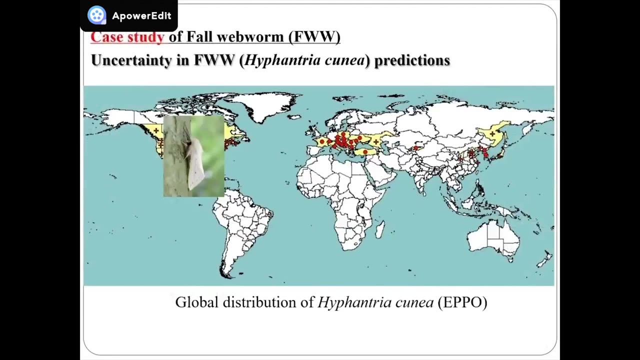 I also compared those model performance based on the omission error and ROC curve, which is very powerful to examine the model performance across multiple thresholds. Let's see the last example. I'm going to use the last example to show the uncertainty in each model prediction and how to use a consistent model approach to overcome those uncertainties. 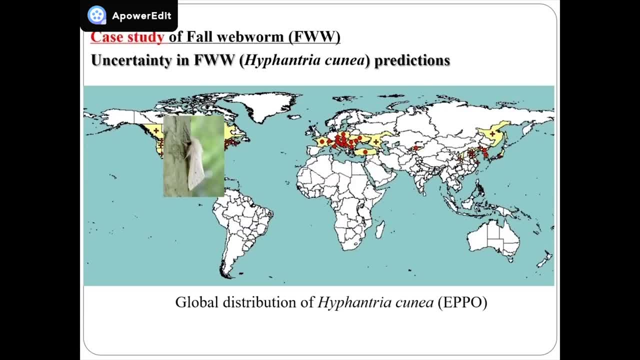 And what's the best method to overcome those uncertainties? So this species is a four-web worm, It's a mouse. It's native to America but become an introduced species in Europe and Eastern Asia. It's not a serious problem in America, but it's a very serious problem in Asia and Europe. 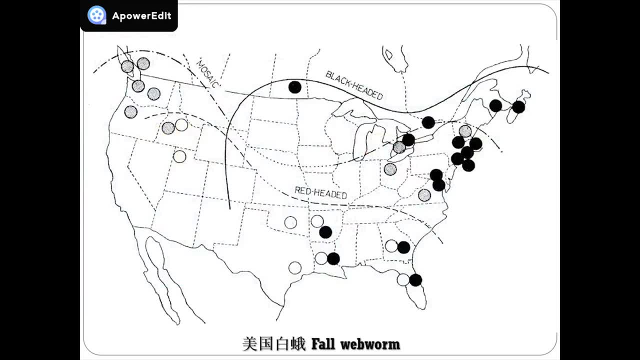 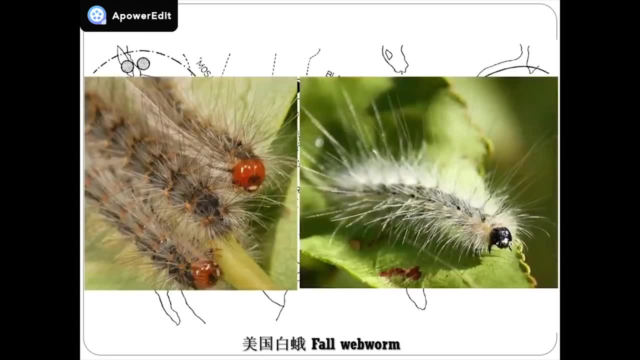 In the native area. there are at least three forms: the black-headed, red-headed and a mosaic of those two-headed. So, but only the red-headed mouses can survive. But only the red-headed mouses can survive. But only the black-headed form had become a introduced species in Europe and Asia. 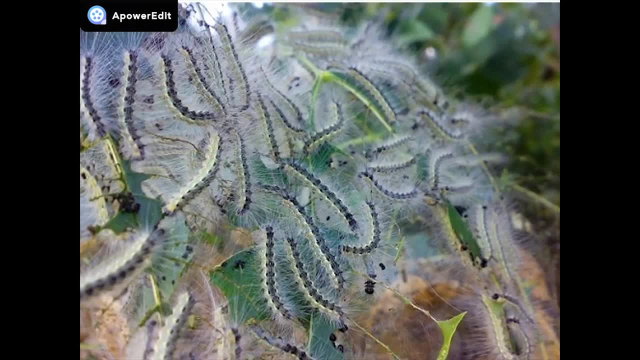 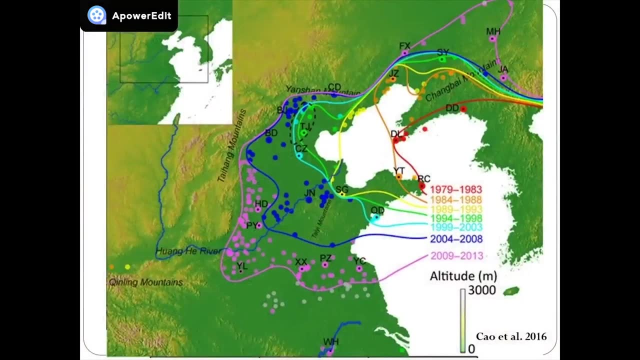 So it's a serious problem in China right now. It's only damaged the broadleaf trees, So it's a very serious problem right now. So here is this figure shows the expselfion of the species in China. It first established the population in the Liaoning province. 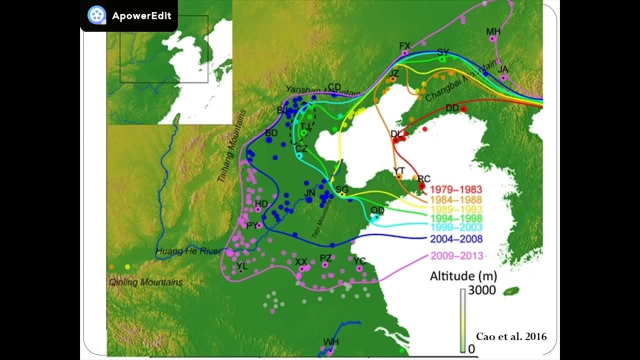 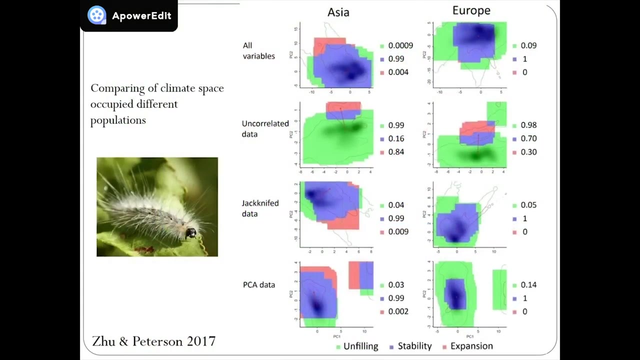 and then after that, expselfion very fast, expansion very fast to the north and south. Currently it seems that this species was blocked. it was blocked the expansion towards the west by the mountains. So here I use four environment datasets. First I compared the climate space occupied by the native 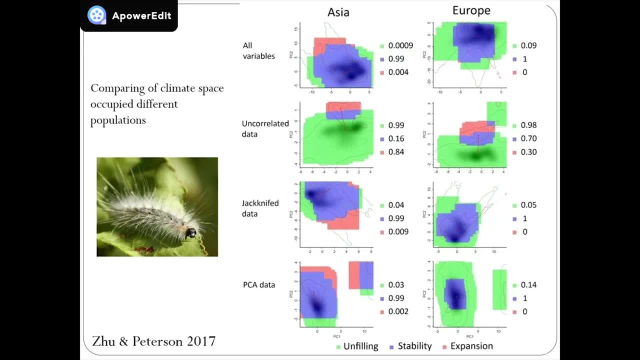 population and introduced population in Asia and Europe. The four environment datasets were included. First, here is all variables, So the first all variables, including those 19 bar kilometer variables. Then the second is uncorrelated variables, by removing those highly correlated variables. The third is JECNF dataset, which selects a subset of those all variables. 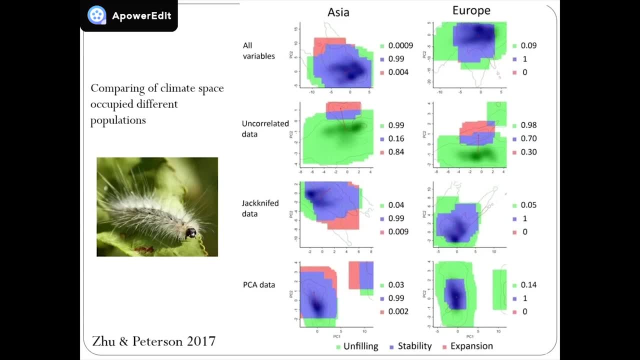 based on the JECNF test of the variable importance, of the variable relevance in species distribution. So the last dataset is PCE dataset. I select the PCE 1 to 5 to select to use for the climate space comparison. So the variables, so the climate space comparisons between native and introduced population, based on 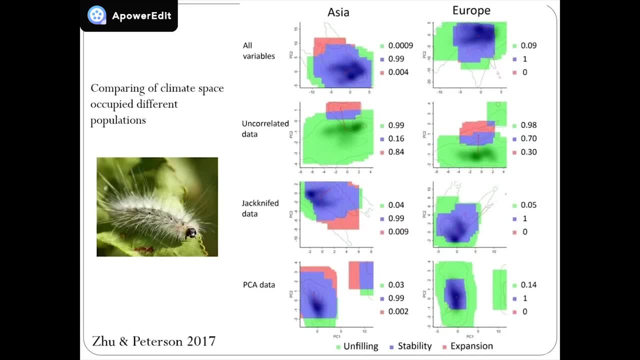 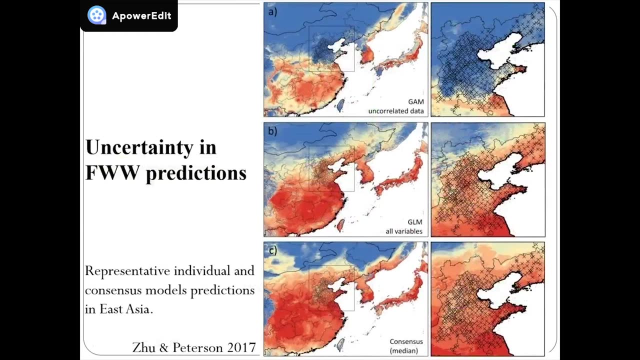 those four datasets. they showed a different degree of niche expansion and niche unfilling. So I use four variable, four datasets and six algorithm, six model approach to generate all the models based on the native area and transferred to eastern Asia. So the more those individual models shows much variety in the 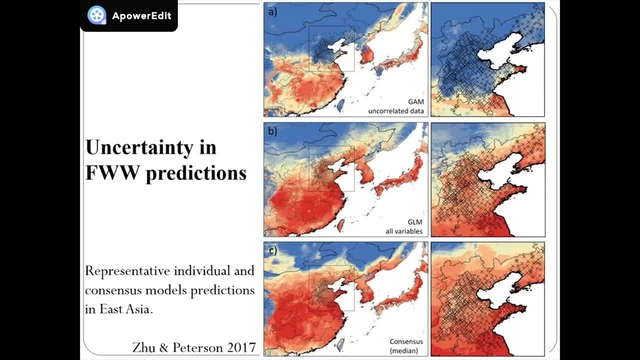 in their ability to capture the introduced point. So the the poorest model that we get is GEM based on the uncorrelated dataset. It failed to capture the points introduced point. The best model we get- i mean the, the model that are show the best transferability- is LM model based on the 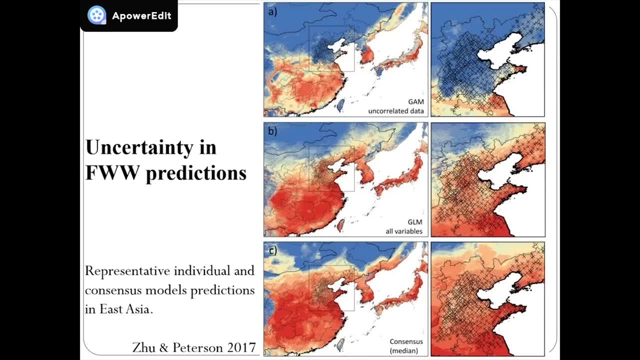 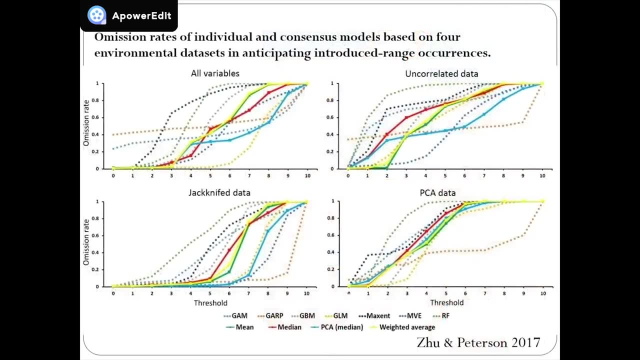 all variables. So the concept's model is seems space, uh, based on it's felt into those two extremes. so I take I take us careful comparison of those individual models. so it seems that the models based on the JECNF dataset showed low emotions. christmas for crossing the time, areャ all. 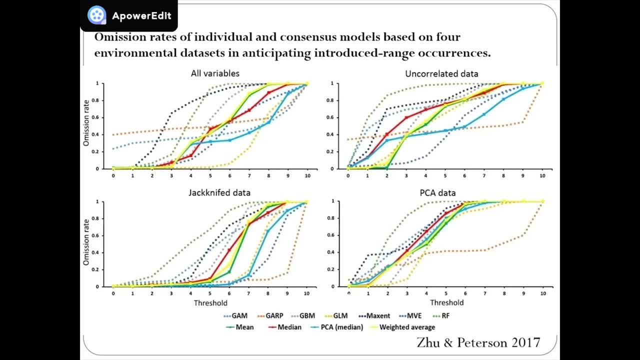 models based on. So it seems that models based on JECNF dataset showed that low emotionphasia in terms ofni번- something limits refer to als reach through the unsparingraw patterns, value when setting the counter punt, etc. the law of motion error compared to those three data sets, which means that it's very important. 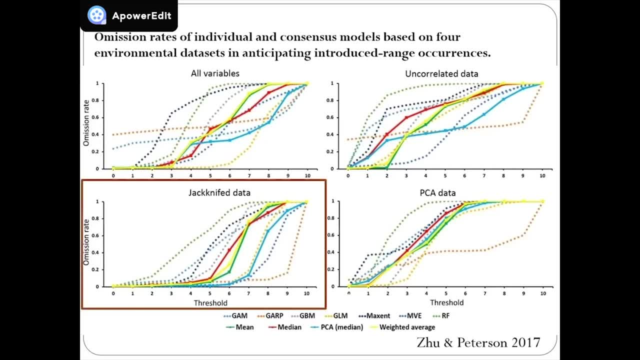 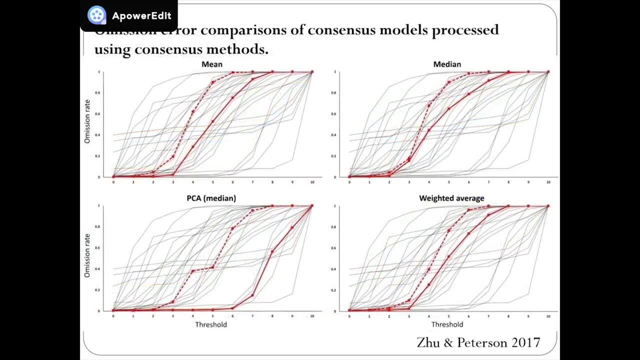 to select the relevant variable, the variable that's controlling the sufficient distribution. I also compared the models that based on the different methods, I mean to generate the constant model. So here is the method that based on, here is the four methods used to generate the. 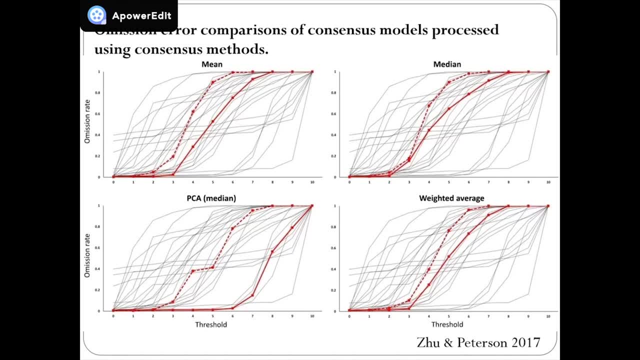 constant model, which is mean media, PCA media and weighted error. If you want to learn how to generate the PCA media approach based on- I mean how to use PCA media approach to generate the constant model, you can take a look at our paper. So from this figure we can 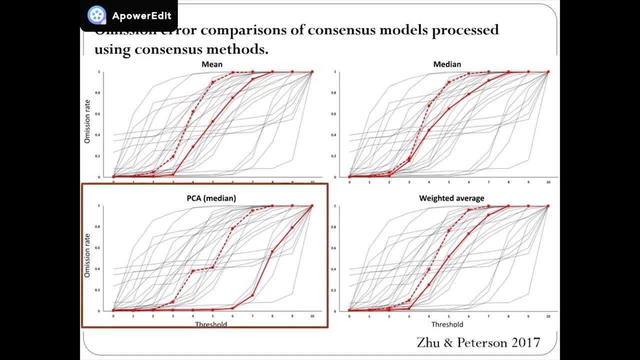 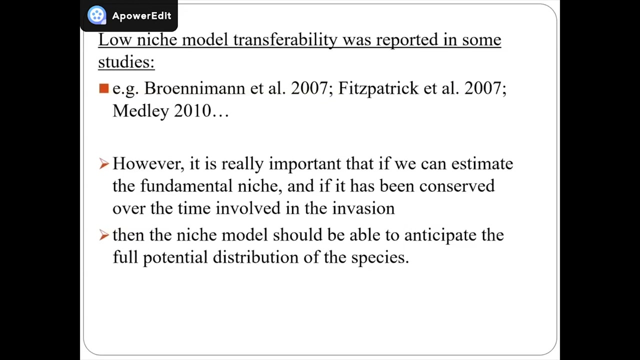 see that a model based on the PCA media approach shows the law of motion error compared to the other approach. Those gray lines indicate the individual model, whereas the red line indicates the constant model based on different subsets of all the individual models. Okay, let's move to the last section: the lessons, the implications of these four case studies. 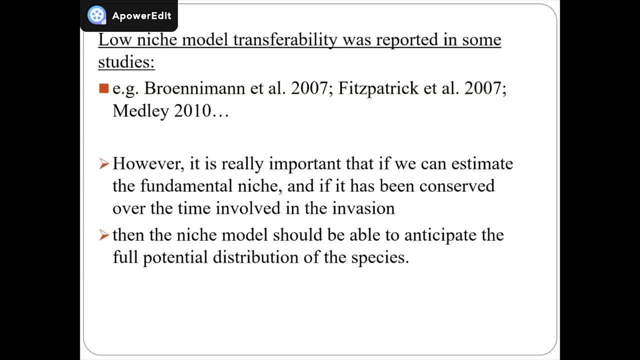 So before that, I want to talk about the low-niche model transferability that was reported in several studies, And there's also also Gates concluding that, based on the low-niche model transferability that they concluded, that niche will shift. However, later research shows that 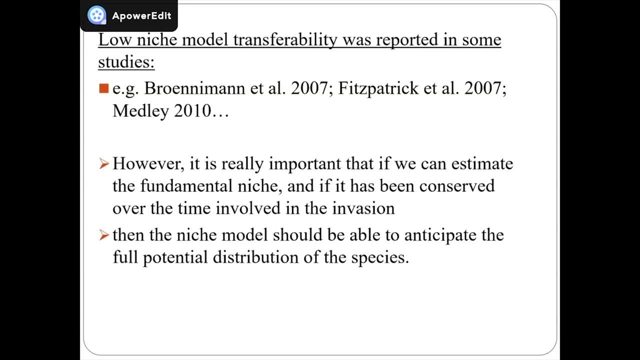 those conclusions are quite artificial. It is mainly because of the environmental datasets. So it's really important that if we can estimate the fundamental niche and if the niche, if that niche had been conserved over the time during the environment process. So this is very important. So all the native niche model approach that should be based 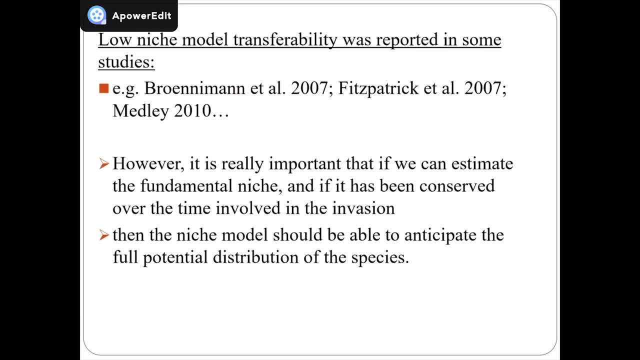 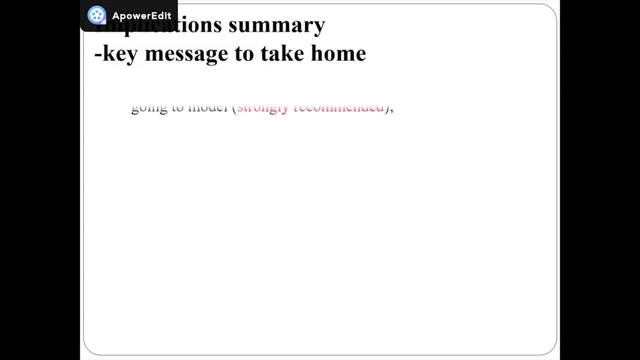 on this hypothesis, Then the niche model should be able to- I mean, anticipate the full partition distribution of the species. It's really important. So the implications are a summary. I would like to outline those points that So. first, 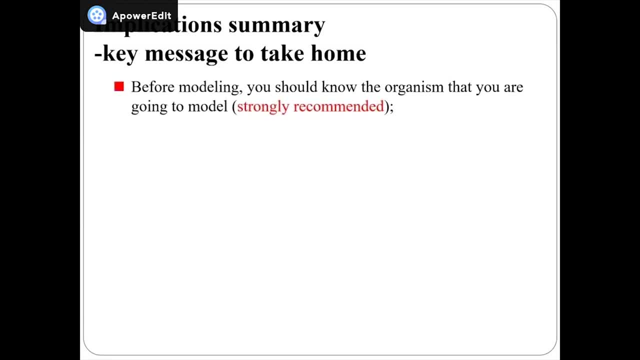 before modeling, you should know the organism that you are going to model. So you should know where they are living, what's the habitat requirement, what's their biogeographical history and- yes, it's really important- you should know the general biology background of the information. 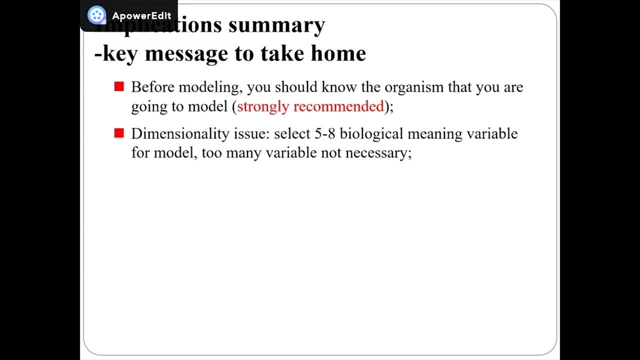 so the dimension and dimension dimensionality issue. that keep in mind. it's better select five to eight variables. too many variables might not necessary. it also can i mean too many variables can lead to a complex model and reduce the model transferability. so it's really important that. 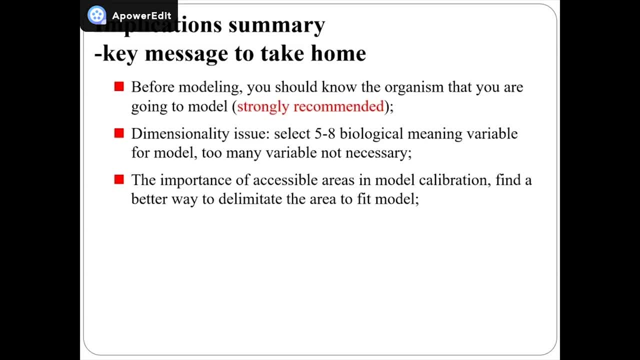 you have to limit this uh, a proper area for your model, because those error reflects whether the species have the partition to move there. so the importance of accessible error in each model collaboration- it's very in. she should be keeping this in mind. i find a better way to delimit this. 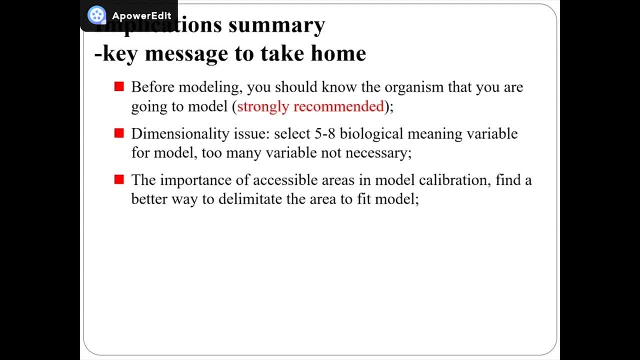 error. so there are several approach available to the limits of the errors. so i would like to recommend you to think of the species in environmental space rather than geographic space, because in environmental space you will know that the response curve the species requirement. uh, why? your model prediction looks like this, but not. 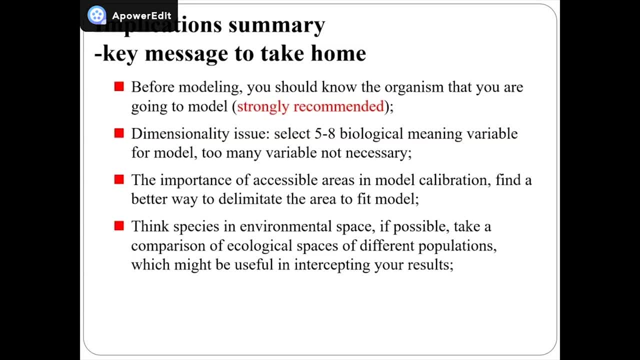 that, so it's real. it's recommended that you take a look at the, the species that uh in environment space, and compare the, the climate space occupied by different populations. the result is very important when you interpret your spatial prediction. so the last- i would last- of this slide, i would recommend you think about the model complexity. 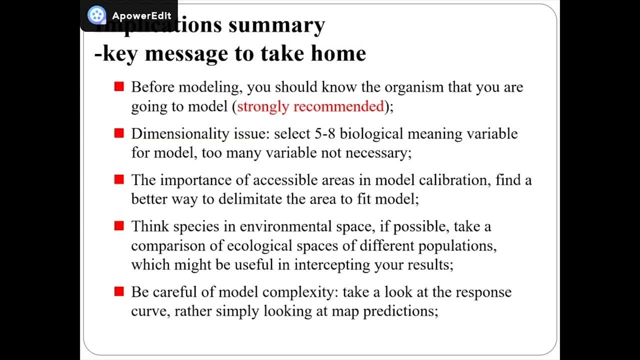 because it's currently it's the most important issue in each model. so take a look at the response curve and the spatial prediction. so what's your response curve looks like? are they smooth or are they? i mean zip code like this. so take a look at the response curve. i mean it's better to before you. 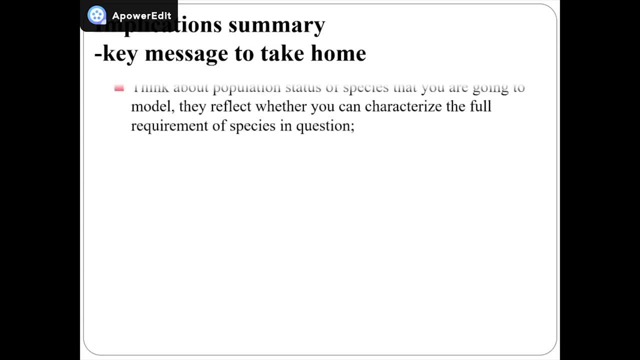 take a look at the spatial prediction. so also, if you think about the population status, whether the species that you are going to model, whether it's stable or it's still expansion, so, because it's the subsharing, each model, application uncertainty. i would like to if you find that, if you're not, 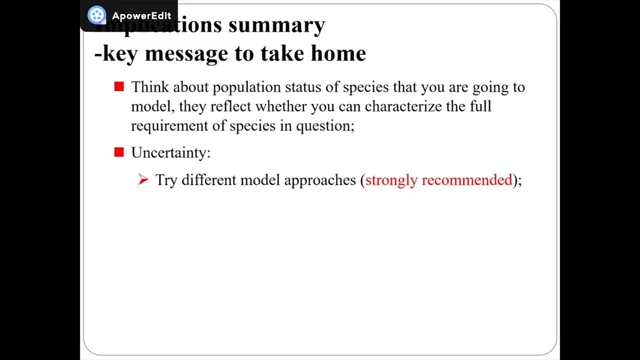 satisfied with your model prediction. i recommend you to try different model approaches, different algorithms, so and see what the model looks like, because they are certain in each model predictions. so you can try individual or consistent model, ensemble mode approach. they have an advantage, disadvantage, but you should care about that. constant models do have. 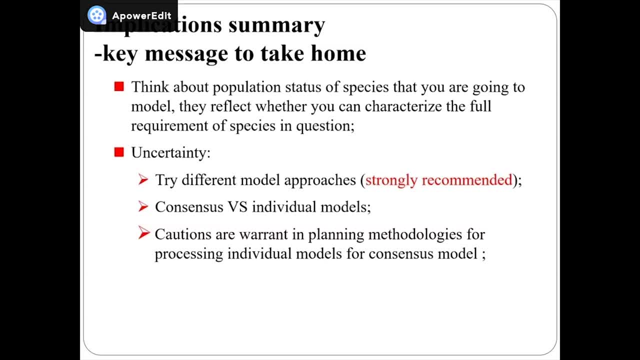 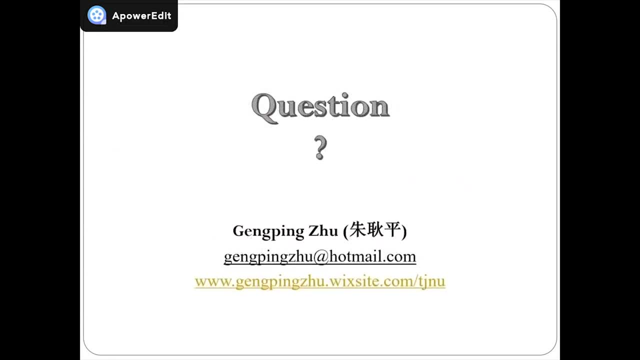 uncertainty, because different methods that yield to produce those constant models. there are also variations among those consistent models. okay, that's it. so if you have some questions, you can. i think you have sent me an email, to me or to this program or to this workshop. i'm happy to answer your question. so that's today's presentation. uh, thank you well. 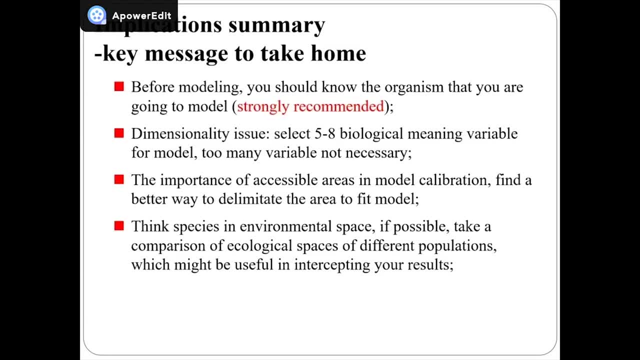 bye-bye uh, in environment space and compare the, the climate space occupied different populations, uh, the result is very important when you interpret your spatial prediction. so the last, i would last, of this slide i would recommend you think about the model. model is a very complex model because it's currently it's a more important issue in each. 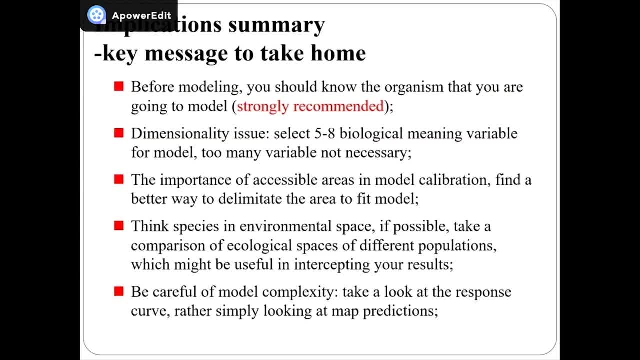 model. so take a look at the response curve rather than simply look at this map predictions. so what your response curve looks like, are these modes or are they? i mean zip code like this? so take a look at the response curve. i mean it's better to before you take a look at the spatial prediction. 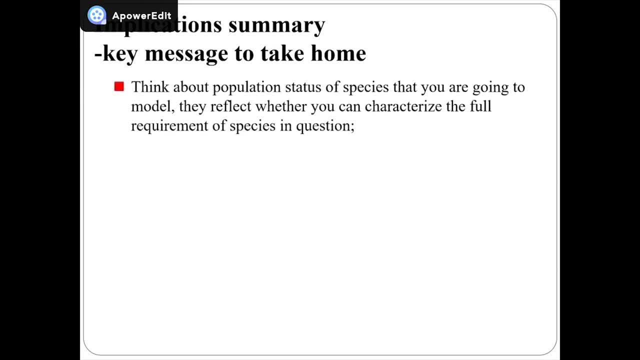 should think about the population data, whether the species data you are going to model, whether it's stable or it's still expunging. so, because it's the case assumption in each model application. On certainty, I would like to if you find that, if you're not satisfied with your model,